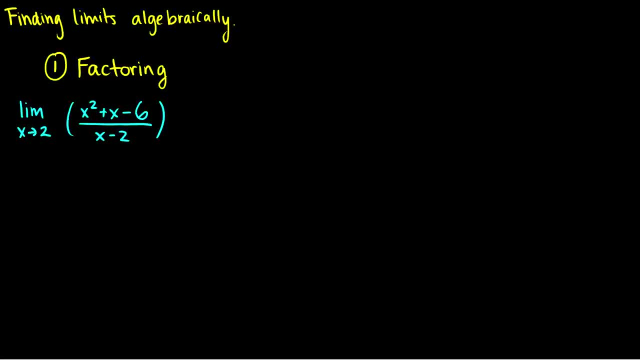 around this. we can factor and hope that something cancels. So let's factor this and factoring is a very important skill. so I highly recommend that if you are kind of rusty on your factoring, you do lots of practice with these limits like an insane amount of practice, Do every question. 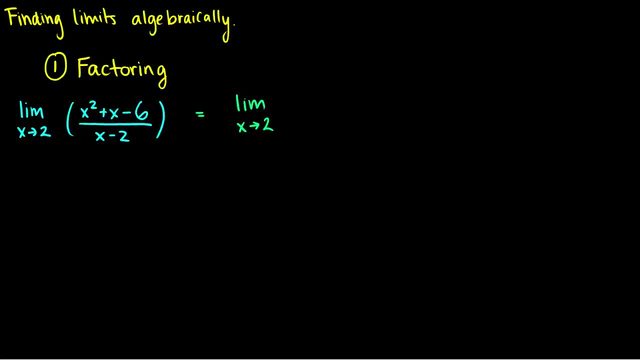 in the textbook you're using if you're rusty on your algebra skills. So x squared plus x minus 6.. How do we factor this? Well, if we have x squared plus x minus 6, we need the last two numbers to multiply to negative 6, and then, when we add them together, they have to add up. 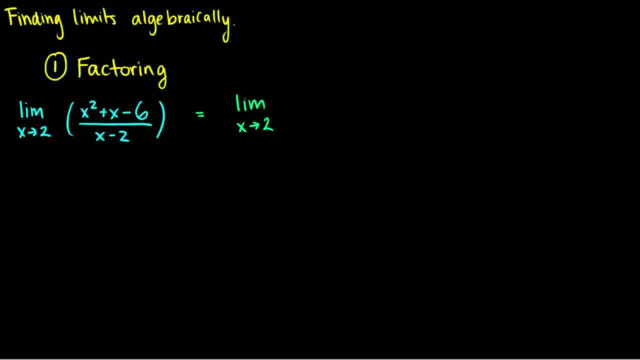 to 1 to get the positive x. So if we factor this, it will just be x plus 3 and x minus 2.. Of course, to make sure that they are the same, we'd have x squared plus 3x minus 2x minus 6, which would 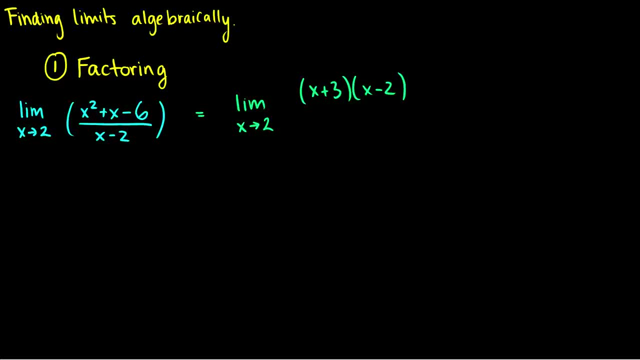 simplify to x squared plus 6 minus or x squared plus x minus 6.. Then on the bottom we still have x minus 2, and at this point we have some luck here, because these can cancel, And then we'll be left with the limit, as x goes to 2, of x plus 3, and at this point we can just substitute x in. 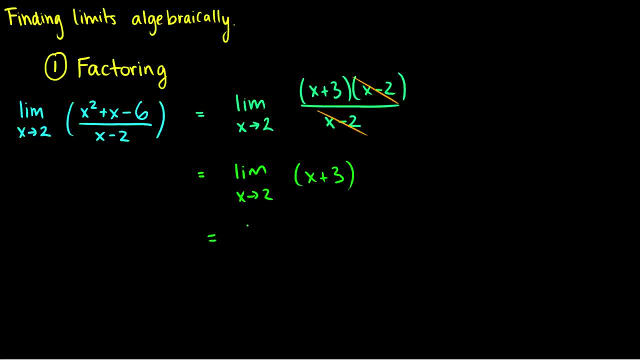 so now we can just say it's 2 plus 3, which is equal to 5.. Now of course these curves aren't the same, so x squared plus x minus 6 over x minus 2 is not the same curve as x plus 3, and this is: 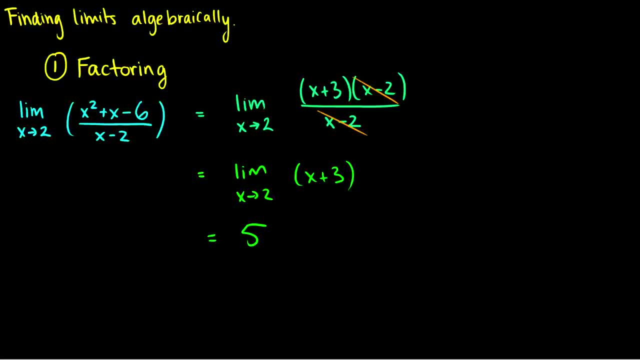 important to note. However, the limits are preserved. so if we graph this, we can see that the limit, as x goes towards 2 of x squared plus x minus 6 over x minus 2, will tend to 5.. However, when we do this- canceling, we are changing the function. That is just a very important thing. 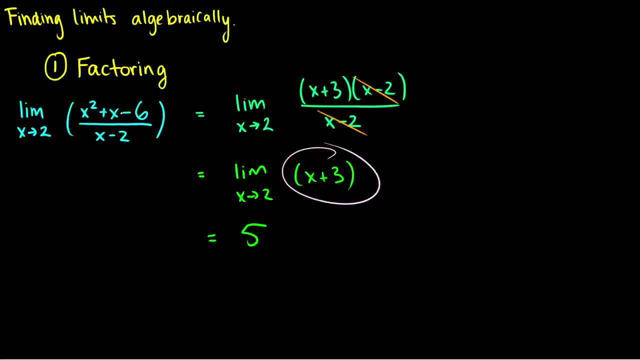 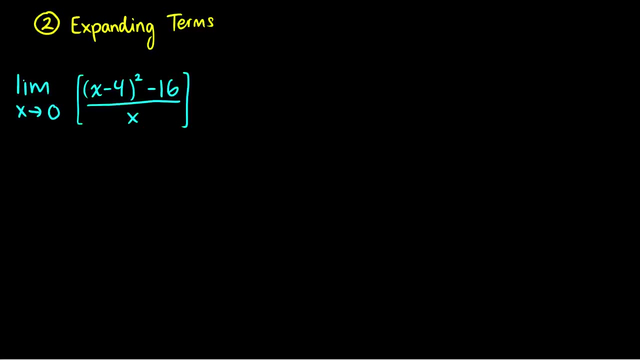 to note. So the limits for these are the same, but the functions are not. The graphs are completely different. So that's factoring. Another method like factoring is just to expand terms. So here we have x minus 4, all squared minus 16 over x, and we want the limit as x goes to 0.. In this, 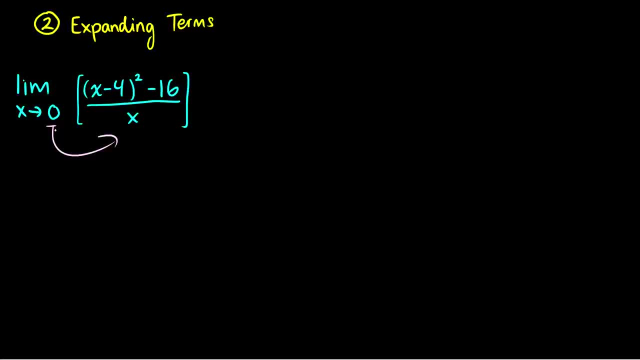 case we have x minus 4, all squared minus 16 over x, and we want the limit as x goes to 0. In this case we can't just plug x equals 0 in, because then we're dividing by 0 again, so we'll have to do. 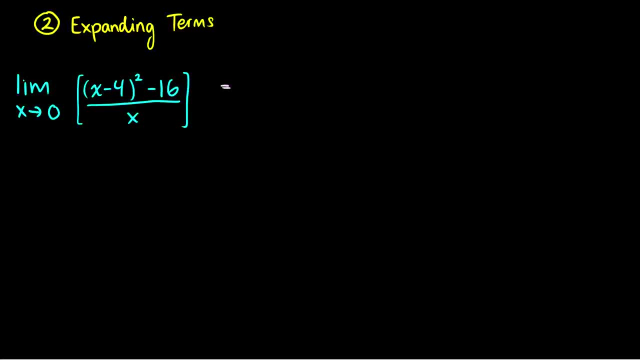 some expanding. So if we expand x minus 4 squared then maybe we'll be able to find something to cancel. We can get rid of that x on the bottom somehow. So the top will be x squared minus 4x minus 4x, so it'll be minus 8x, and then negative 4 times negative. 4 is positive 16. 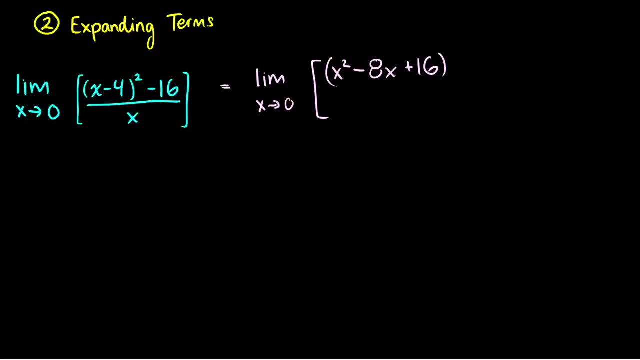 so we have all that After we expand it out, then we subtract 16 and then we divide by x. Okay, this looks like maybe something we can work with, so let's simplify as much as we can The limit. as x goes to 0 of well, this will be x squared minus 8x, and the plus 16 and minus 16 cancel each other. 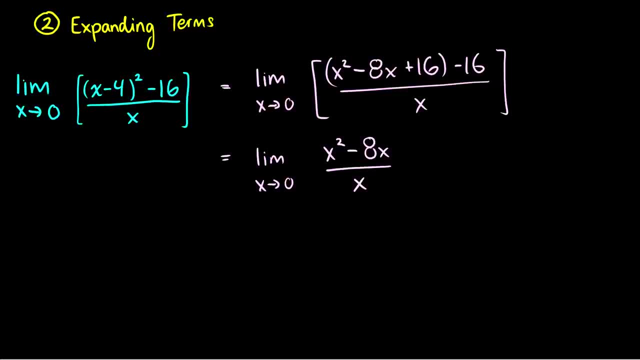 out. so that's good, And we have x on the bottom. Oh, what do we have here? Well, now we can cancel an x from the top and bottom, so we can divide the top and bottom by x, and we'll be left with: so, essentially, cancel these out. we'll then be left with the limit as x goes to. 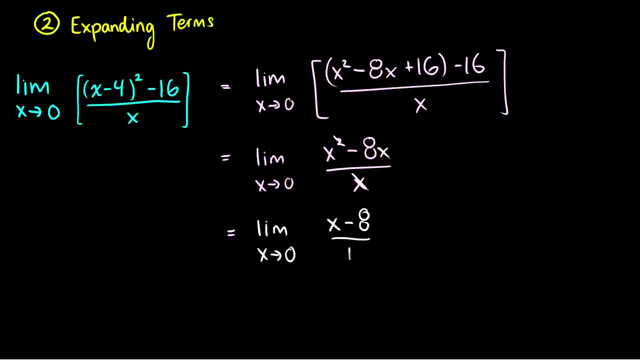 0 of x minus 8 over 1, which just simplifies to x minus 8, and then if we plug 0 in for x, we'll have 0 minus 8, which is just equal to negative 8.. So by expanding terms we were able to cancel out that x on the bottom and find the limit Again. I 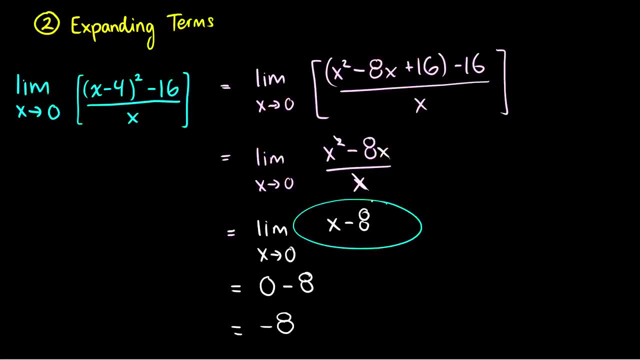 have to really emphasize that of course, x minus 8 is not the same diagram as x minus 4, squared minus 16 over x. They're different graphs, they're different functions, but their limits happen to be the same. So that's expanding terms, The most complicated trick that everyone is. 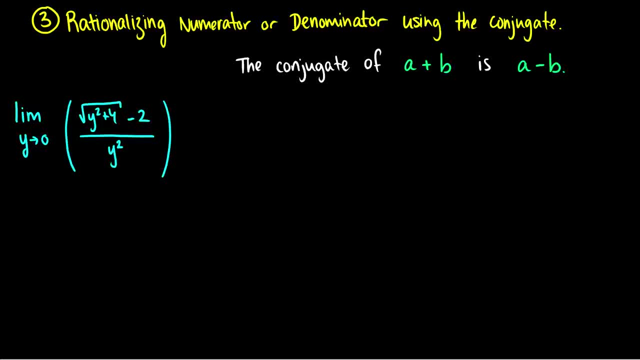 confused by in their introduction calculus course, because they never really practiced this in high school- is rationalizing numerators or denominators using the conjugate. So here we have: y goes to 0.. There's nothing to expand, there's nothing to factor, but I have to. 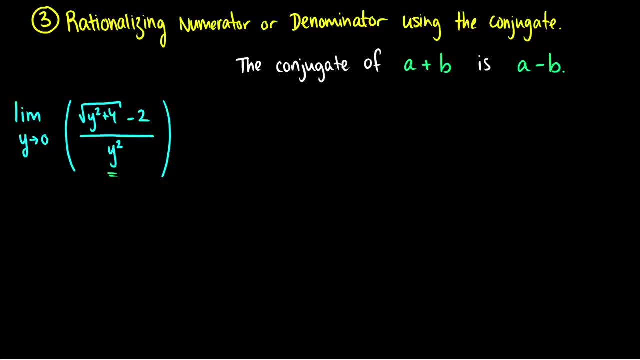 get rid of this y squared on the bottom in order to plug in a limit. So what do I do? Well, essentially, I want to multiply the whole thing by 1.. Now, just multiplying by 1 on its own isn't very helpful, but if we multiply by 1 where we use the conjugate of a term, 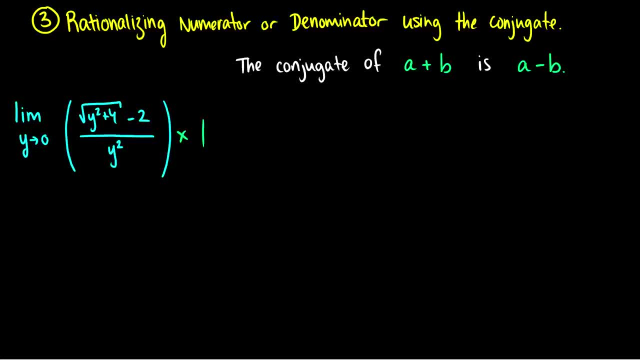 we already have, then maybe things will look nicer. So what is a conjugate? Well, if we have some a plus b, then the conjugate is just a minus b. So what happens when we take x minus a and we multiply by the conjugate x plus a? What 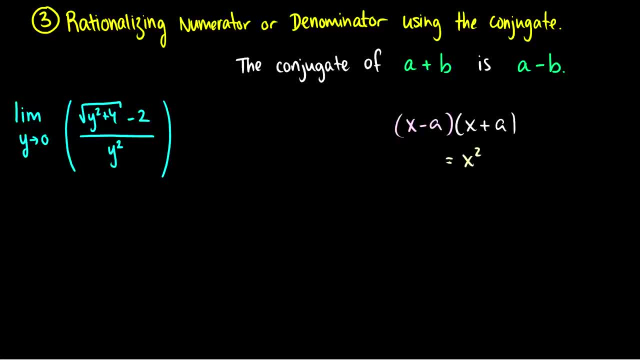 nice thing happens here. Well, we end up with x squared Minus ax plus ax plus a squared, which just gives us x squared. Sorry, this should be minus a squared, so should be x squared minus a squared. So that's nice. So if we take a look at our square root of y squared plus 4 minus 2 over y squared, 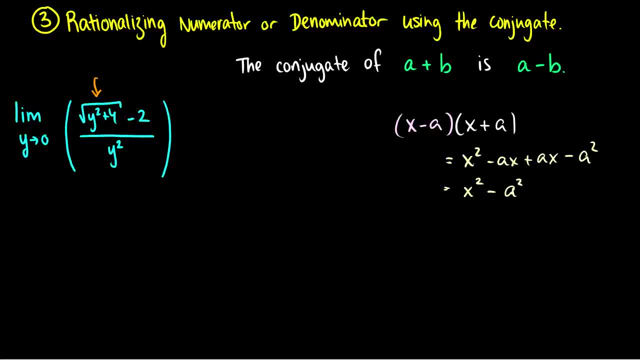 this term here is a square root, But if I multiply by the conjugate then I'll be able to square it. And if I can square it, that means that I can cancel out that y squared on the bottom. So let's do this, Let's multiply by the conjugate. Now, how do we form the conjugate? 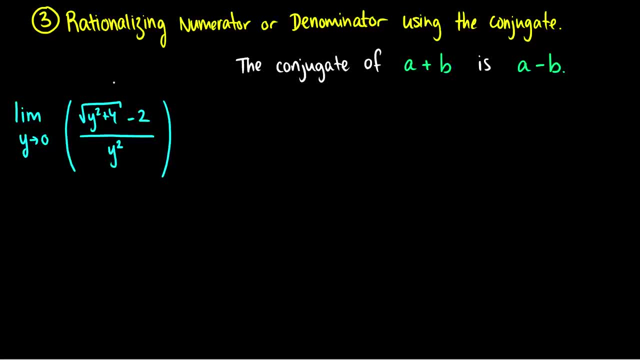 Well, we take two terms, we'll call them a and b, and this would be a minus b in this case. So we just multiply by a plus b, So that'd be the square root of y squared plus 4.. And then we add 2.. 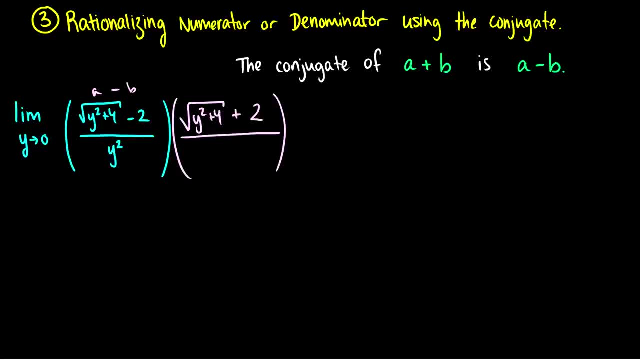 Instead of subtracting 2.. So that's the conjugate, And of course we have to multiply the whole thing by 1.. So that's where this trick comes in: We just multiply the top and bottom by the same thing, and this is just the same as multiplying by 1.. 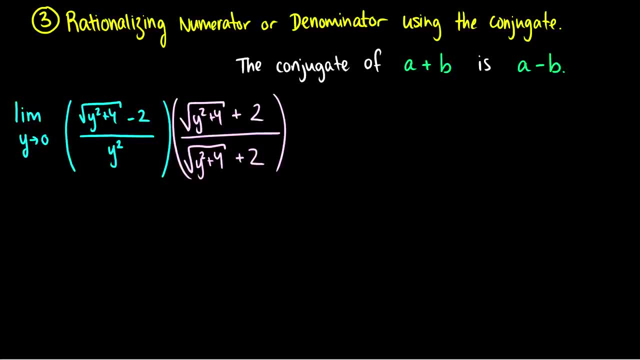 Okay. so now that we've multiplied by 1 with a really fancy method, we can then multiply these out and maybe get a nicer limit. So I said before that if we take x minus a times x plus a, we'll get x squared minus a squared, So we don't really need 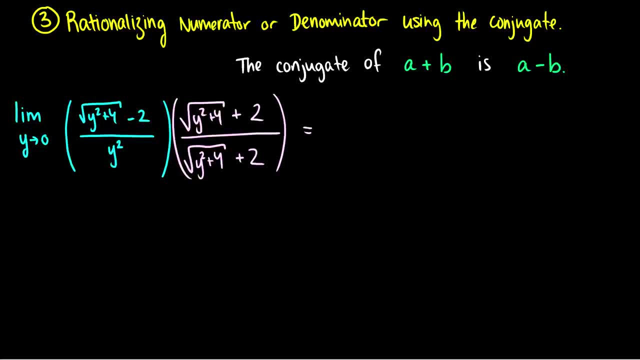 to take all the terms on top, because we know that if this is our x and we multiply them together, we're going to get x squared. So on the top we're going to end up with y squared plus 4.. And if this is minus a and this is plus a, We're going to get minus a squared. 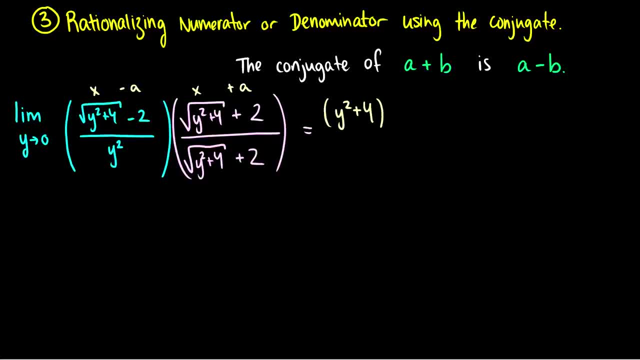 So what is a? a is 2.. What is a squared two? well, 2 squared is 4, and we're going to end up with minus 4, because we're going to end up with minus a squared. so now we have y squared plus 4, minus 4 on the top and then on the bottom. 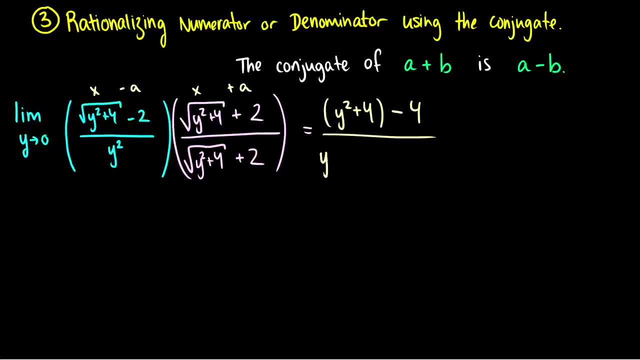 well, we just multiply them together. so we're going to have y squared on its own, and this will be multiplied by the square root of y squared plus 4 plus 2. now this ugly thing is still going to be on the bottom. we're just going to hope that it doesn't cause a problem. for. 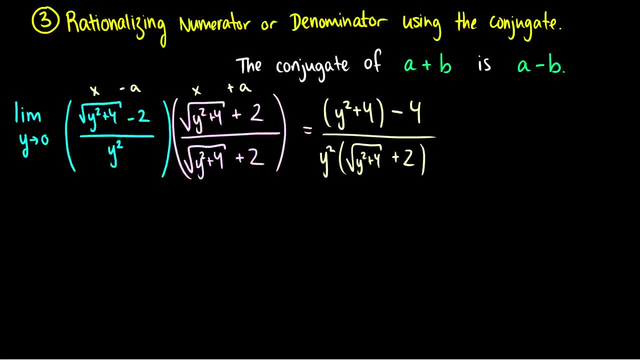 us, and of course i really should be consistent and say that: right, this is in fact the limit, as y goes to 0 of y squared plus 4 minus 4 over y squared times the square root of y squared plus 4 plus 2. so we can simplify a little bit on the top: the plus 4 and minus 4 will cancel out. 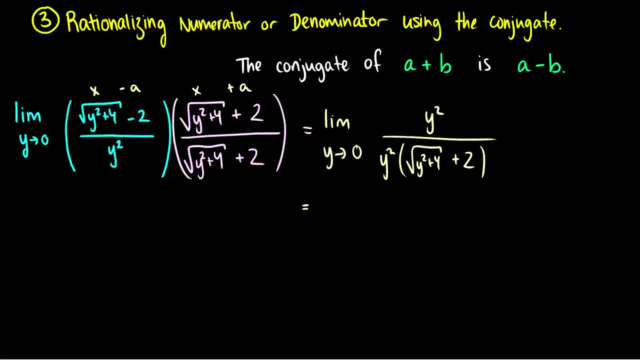 and we'll just be left with y squared. so so now, at this point, we can cancel out these y squareds. and what are we left with? well, we're left with the limit, as y goes to 0, of 1 over the square root of y squared plus 4 plus 2. 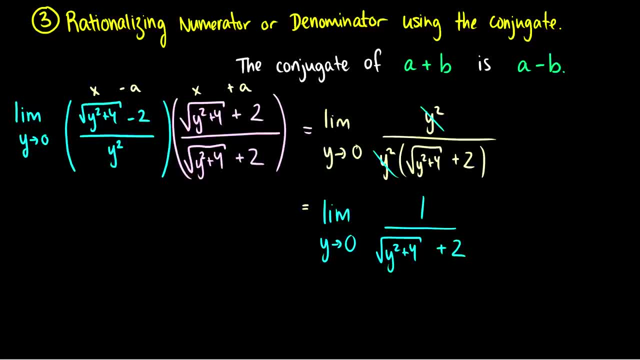 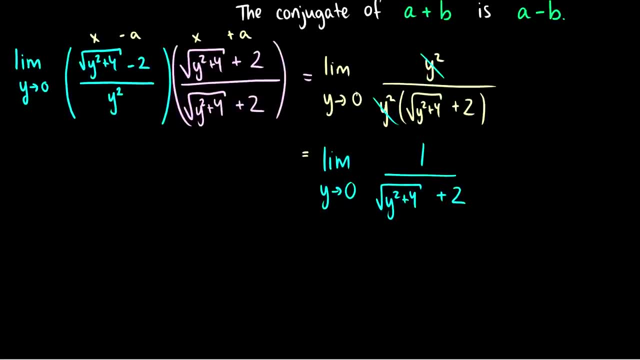 now. this is nicer because we can plug in: y equals 0 now, because if we do, we're not going to get 0 in the denominator anymore. so if we plug in 0, this is one over the square root of zero plus four plus two, which is just one over the square root of four. 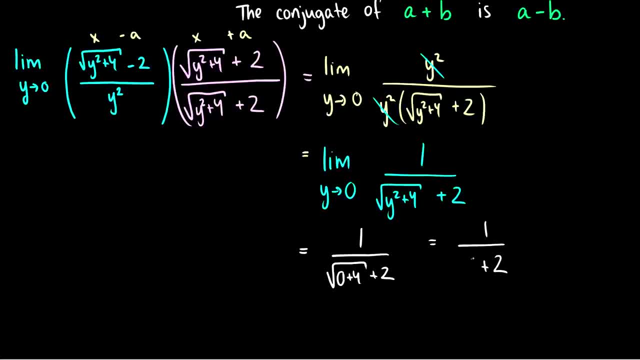 plus two, and of course the square root of four is just two. this is one over two plus two, which is just one over four. so the limit of this nasty thing is just one fourth, and by using the conjugate essentially multiplying by one, we're able to turn it into a form that we can reduce. 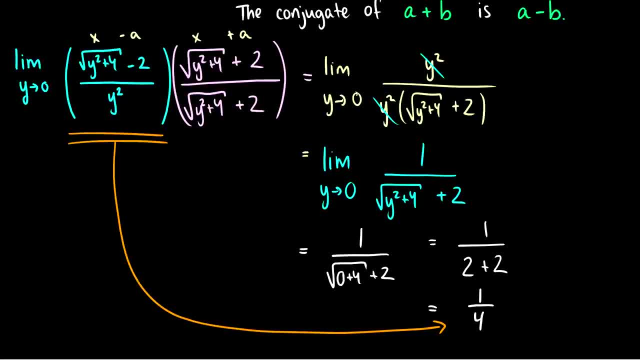 and then get a value out of. of course, with a graph we could see very clearly that the limit was one fourth, but just looking at it algebraically it's very hard to tell. so using these mathematical tricks and methods, we can get something we can work with. okay. so those are. 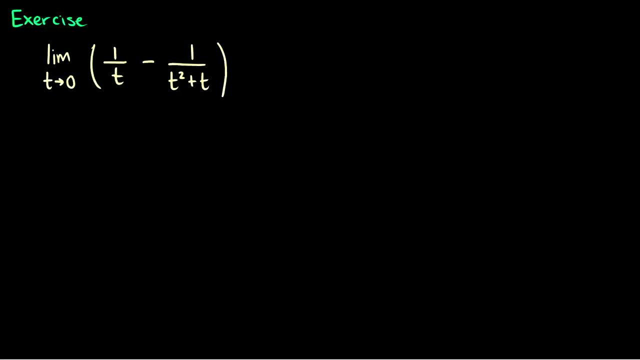 three really important tricks. in fact, they're not even tricks, they're methods. so let's do an exercise or two and practice some more. so here i have the limit, as t goes to zero, of one over t minus one over t squared plus t. of course we can't just plug in zero, because then we're left with one over zero. 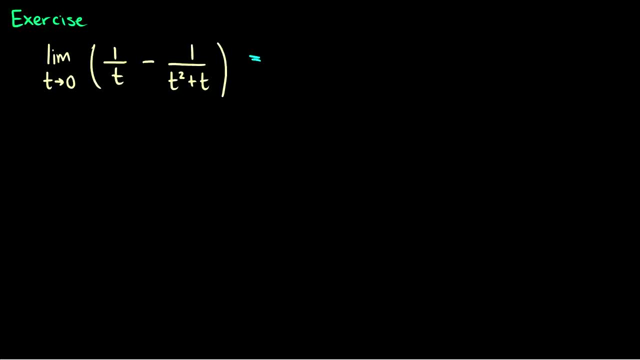 in both cases. so here's another trick you might have forgotten, which isn't even a trick. i shouldn't call them tricks, because these are just methods. they're not tricks. they are methods that you should know. well, let's factor some things first and see if we can find a common denominator. 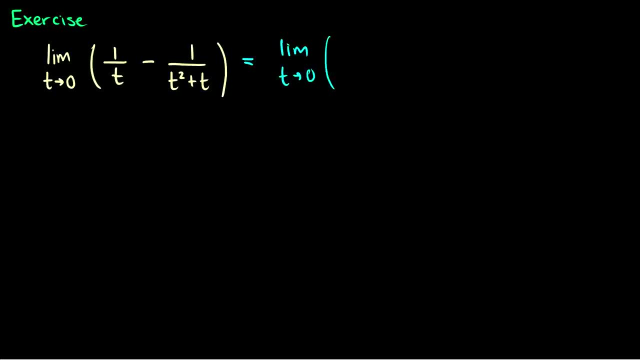 so this would be the limit, as t goes to zero, of well, one over t we can't really do much with, but we can subtract one over and we can pull out a t. this will be t times t plus one. okay, so we can find a common denominator. 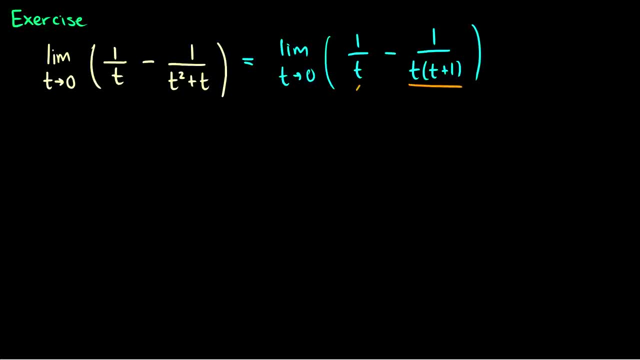 and our common denominator will be t times t plus one. so we should just multiply this one over t by t plus one and then we can put them together. so again more just subtraction and addition with fractions. again, you should probably review this if you don't quite remember. but just 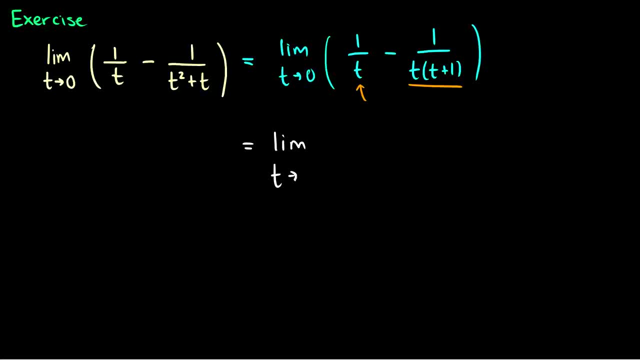 to show the steps here. so the limit as t goes to zero. we need a common denominator so we can multiply by t times t plus 1. in fact we can just multiply everything by the common denominator, so we can say this is 1 times t times t plus 1, and this will be the limit with, at rule: times t plus 1. 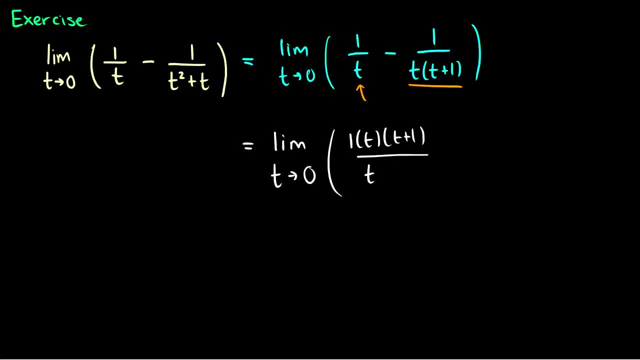 t times. I said it'll be times t, and then we subtract, well, we multiply that t times t plus 1, and then we'll end up with: well, it'll cancel, so it'll be just minus 1 on top, In fact, maybe I. 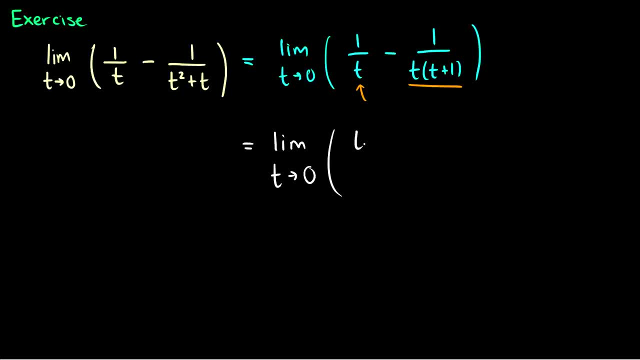 should just simplify this right away. So essentially we'll end up with t plus 1 over t times t plus 1, which is the common denominator, and then we subtract the 1 originally. So essentially we just multiply by whatever is not common. So we have t already, so we just take the t plus 1,. 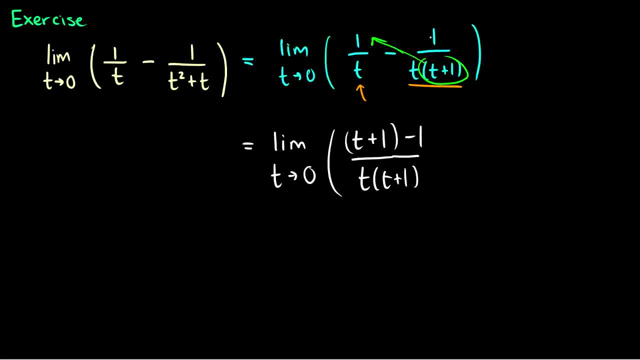 we multiply it by the 1, we already have t and t plus 1 on the right side, so we just keep the 1 there. Okay, and now we can simplify a little bit. So this is the limit as t goes to 0 of. 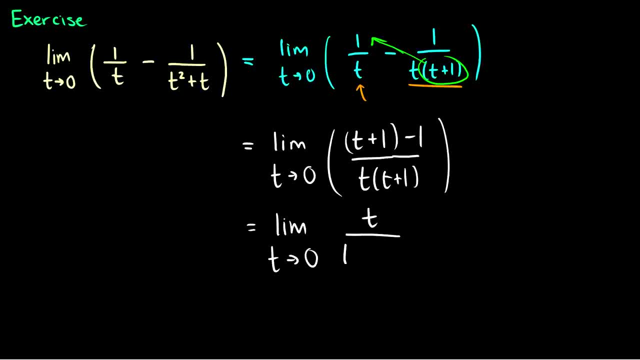 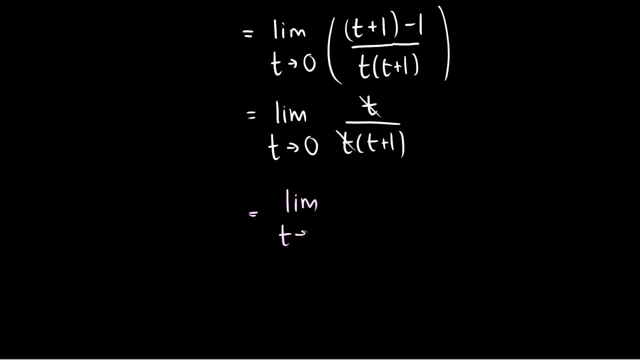 well, t plus 1 minus 1 is just t and this is all over t t times t plus 1, and I see something really nice here. I see that I can cancel these t's out. So now we have the limit, as t goes to 0, of 1 over t plus 1.. We can now just plug in 0 for t. 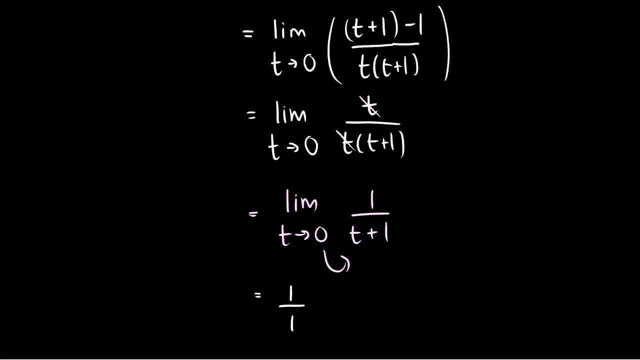 and we'll get that. this is just 1 over 1, which is just equal to 1.. Okay, so again another skill you should be able to do, which is working with fractions and simplifying it to get a limit that you can deal with. One more, The limit as x goes to. 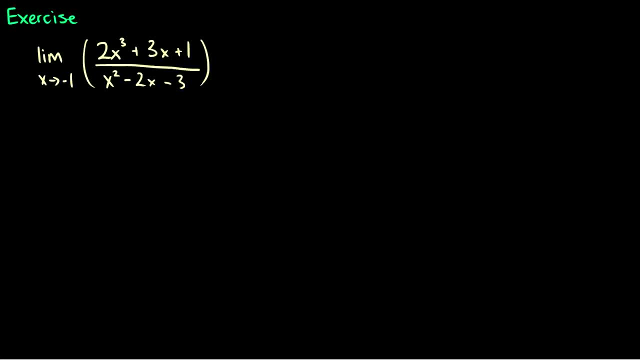 negative 1 of 2x cubed plus 3x plus 1 over x squared minus 2x minus 3.. What do you think we have to do here? Well, we definitely have to factor these. So let's begin by factoring the top and the bottom. and oh, this is going to be so much fun to factor. So 2x cubed. 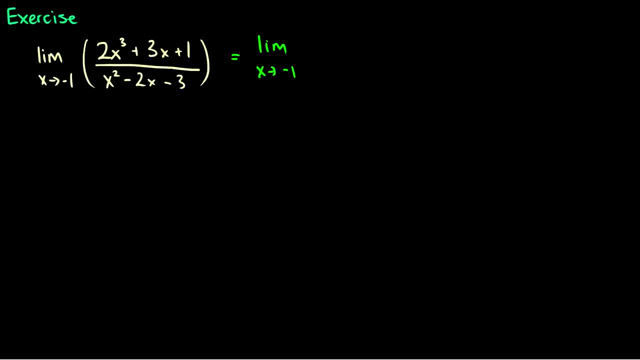 plus 3x plus 1.. Our constant should multiply together to get 1.. It should add together to get 3.. So this looks like it's going to be 2x plus 1 multiplied by x plus 1. when we factor, We can multiply these out to: 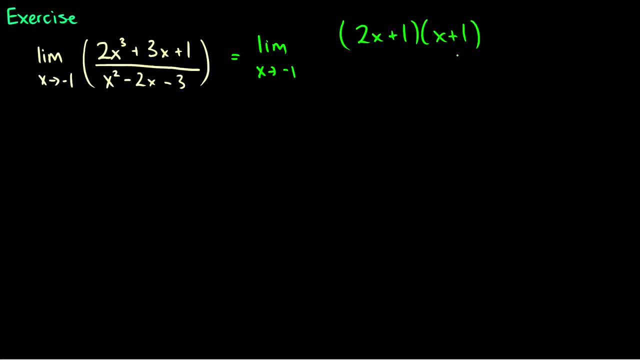 check for sure. So it'd be 2x squared plus 2x plus x, which is 3x plus 1 times 1, which is 1.. So that works. And then of course the bottom would be x minus 3x plus 1..